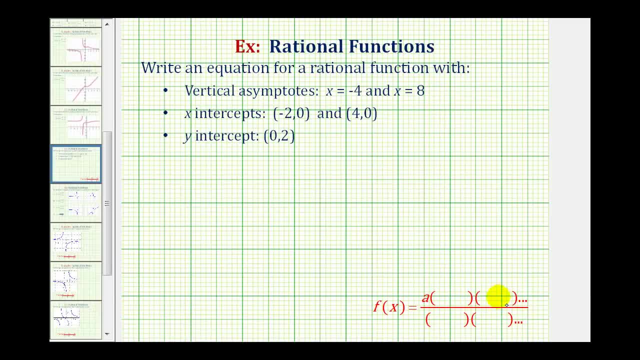 where a is a constant and we'll have factors in the numerator and factors in the denominator. Knowing the vertical asymptotes of a rational function gives us information about the factors in the denominator. Knowing the x intercepts of a rational function gives us information about the factors in the numerator. 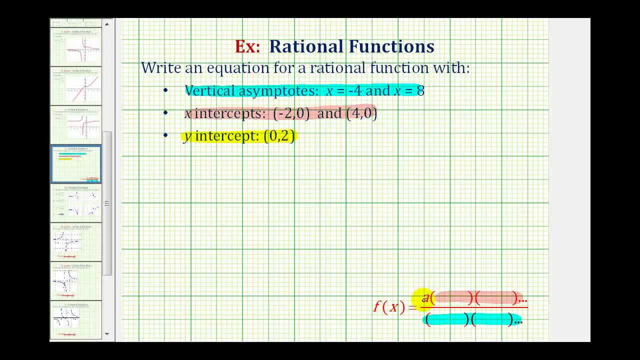 And then, using the y intercept, we can determine the value of the constant a. So let's go ahead and see if we can set this up. We'll have f of x equals. we'll have to find a in the second step, and now, because we're given the vertical asymptotes. 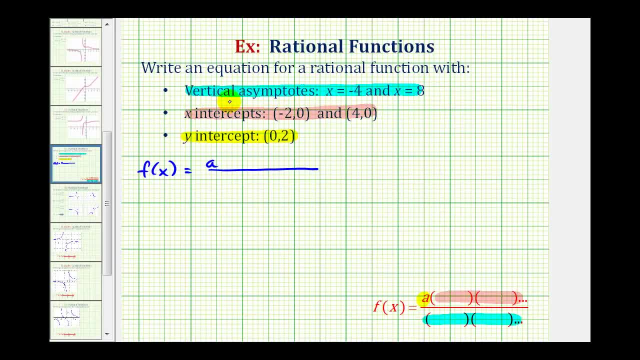 are x equals negative four and x equals eight. remember these values are found by determining where the denominator is equal to zero. So if x equals negative four is the equation of a vertical asymptote, then one of the factors of the denominator must be x plus four. 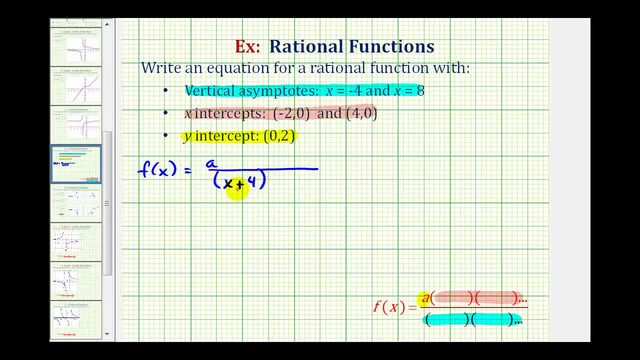 Notice how negative four is a zero of this factor, or makes this factor equal to zero. And if x equals eight is a vertical asymptote, then x minus eight must be a factor of the denominator. Next, we're told, the x intercepts. 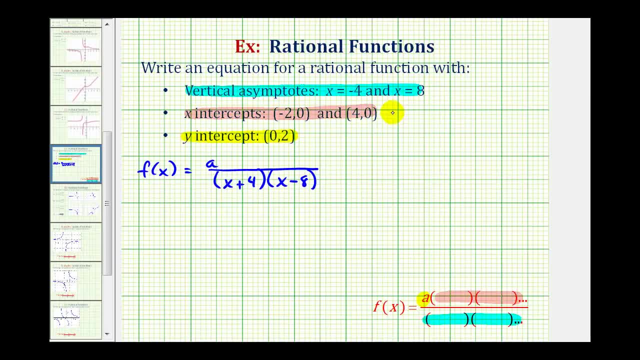 our negative two and positive four. Remember this is telling us that f of negative two equals zero and f of four is equal to zero. So these are the values where the function is equal to zero. A rational function is equal to zero when the numerator is equal to zero. 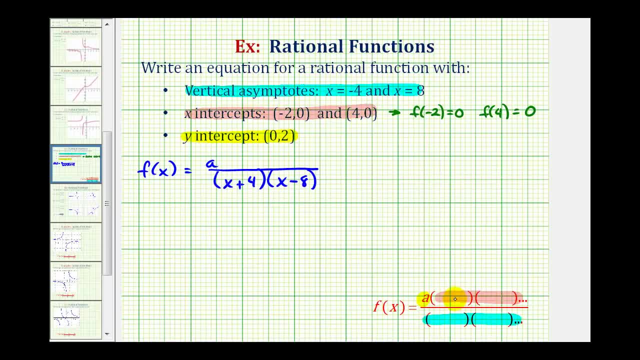 So if negative two makes the function equal to zero, then the numerator must have a factor of x plus two. And if x equals four makes the function equal to zero, then x minus four must be a factor in the numerator. Now the last thing to do is find the value of a. 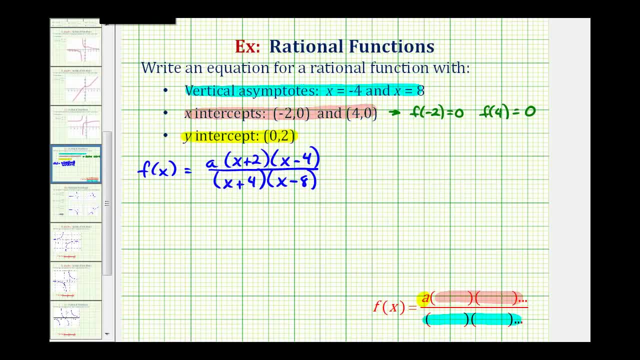 and we can do this using the y-intercept. If the y-intercept is the point zero two, that's telling us that f of zero must equal two. So we can substitute zero for x, set the function value equal to two and solve for a.